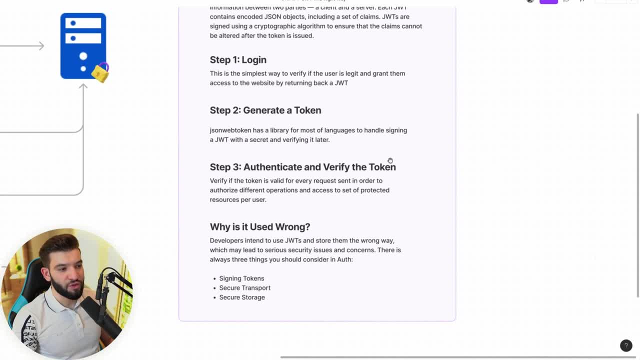 for us pretty well And once we got the GWT and once the user wants to access something, he can authenticate And of course we're going to verify that particular token. So this is a basic block verification of the token. Now I want to go deeply into why is it used wrongly and what is? 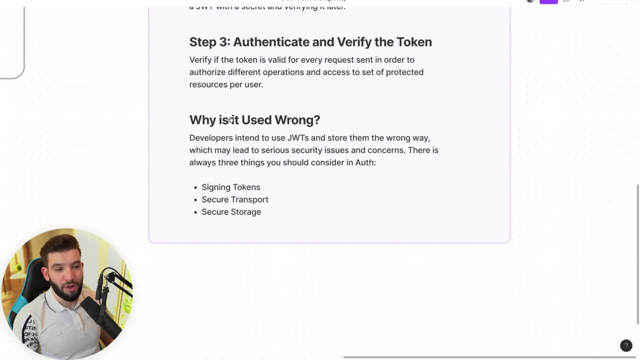 going on wrong with this particular way and how you should probably secure this and how you should think about it. So if we take a look on GWTs, they are just tokens and they allow you to use those tokens in a stateless way. That means you don't need to keep states on the server side And that's. 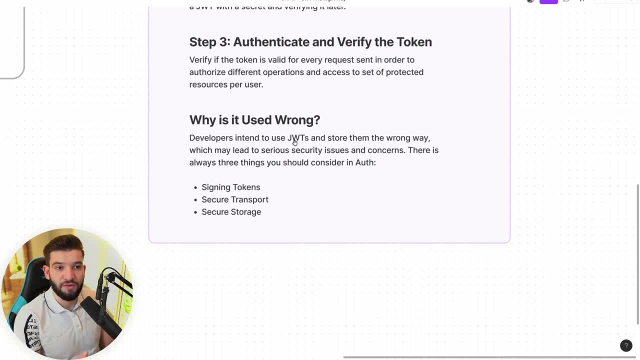 why GWTs exist. That's why they just keep this particular payload. that keeps, for example, the user ID that is currently authenticated and everything, And of course, they are encrypted, and so one thing or like, there's always three things that you should consider in authentication. 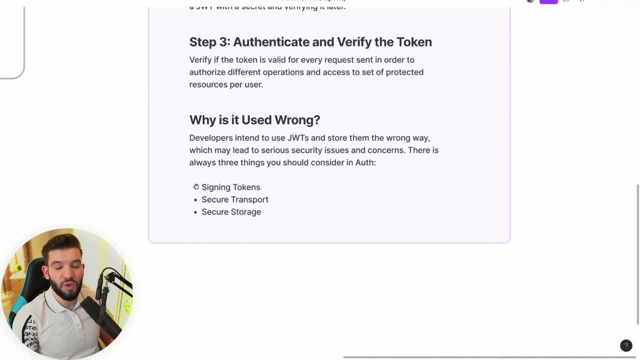 Signing tokens means encrypting the tokens and making sure the token's data is not accessible by anyone on only your server or yourself. You need to have a secure transport And this, of course, this can be happening just like an HTTPS or using SSL, So make sure to do that. 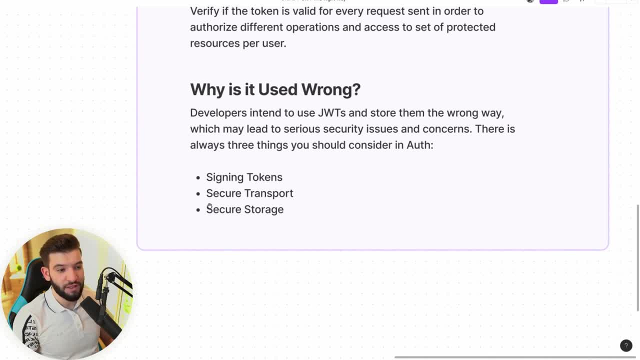 And last but not least, which is the most vulnerable part of all of this, is securing the storage, And what I mean by screen storage is actually putting or saving those GWTs in a secure place, because if you don't save them in a secure place, you're going to have, you know, a lot of pitfalls and a lot of issues regarding. 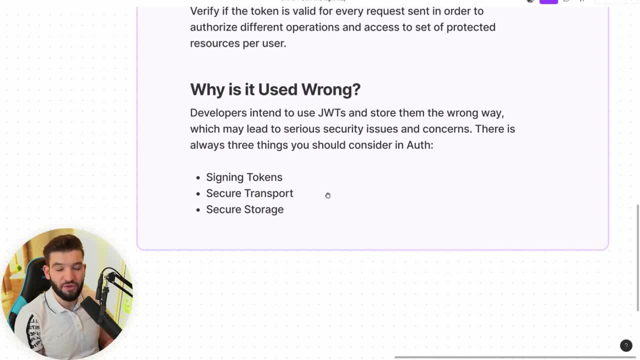 that And you're going to allow, like side parties, will allow hackers or anybody else with bad intentions to use those GWTs of your users and to actually access their resource on behalf, And it can do plenty of stuff like from XSS to CSRF and session hijacking and plenty of. 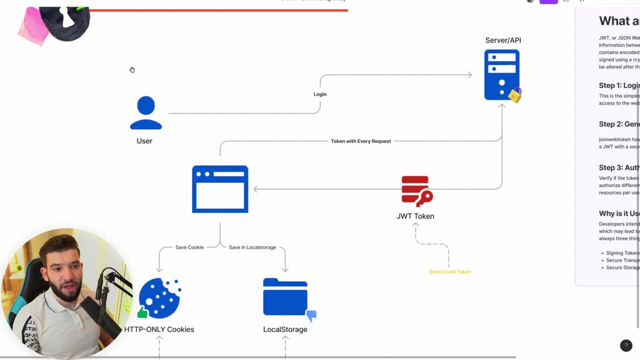 stuff that you don't want to have. On the other hand, if we jump into the diagram like a user who wants to log into a server, he basically just, of course, logs into the server. the server is going to send back the GWT token, is going to sign the token and 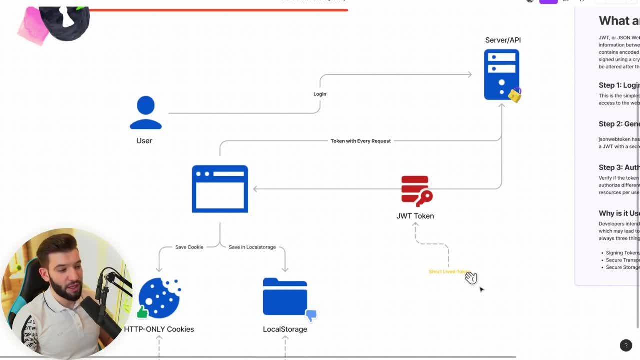 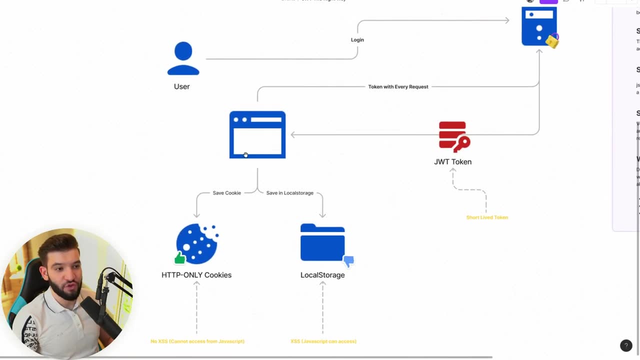 everything, And this is just going to be a short lived token, So like it has a pretty small expiry date And that's that's. that's one point I want to talk about. So once you've got the token in here, the browser needs to handle storing the token so it can send that token with every. 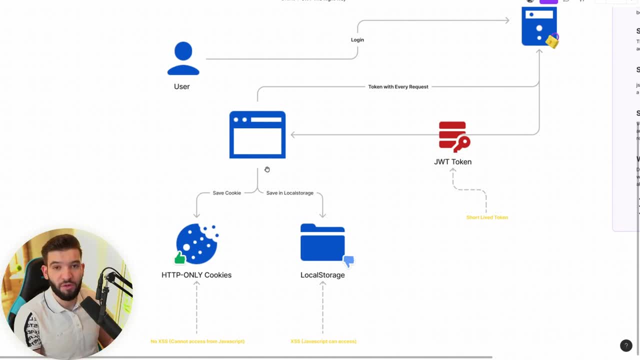 request made after login. So you know you can to allow basically users to authorize after login, you have to send that token until server a. I got this particular token, I can access this particular resources and they have the authority to do so. So for that, particularly what happens, you can actually save it into two. 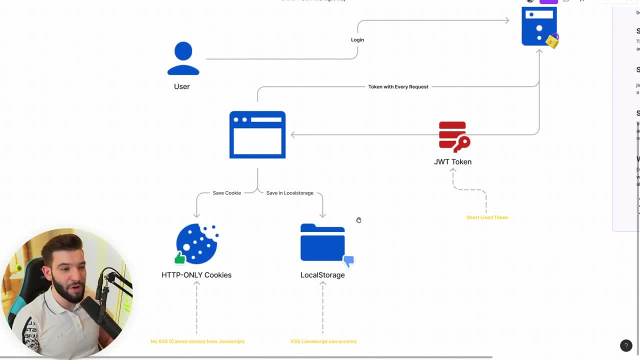 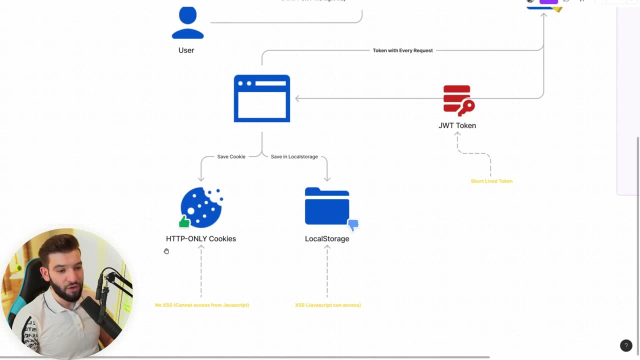 places. One is the local storage, which is the easiest and the most simple place, But still it's actually so vulnerable And it's so bad practices. storage on a local storage And you can do it on cookies, and particularly HTTP only cookies. So you can save them in two places: in 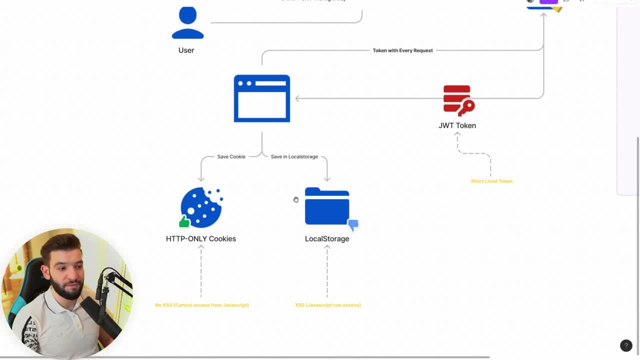 here And I'm going to give you this- I can this particular video, an example between a difference between storing to the local storage and what are the vulnerabilities from XSS to a CSRF that's going to, you know, just going to expose your server when you do it on local storage versus when you do it on HTTP only cookies. 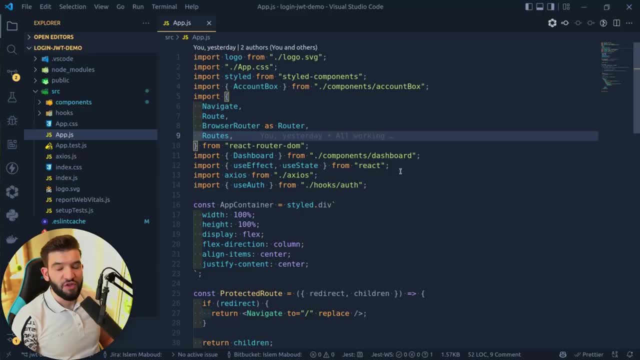 and why the benefits or what are the benefits in this particular? So for our demo projects in here we got actually two projects. we got the front end project which runs react and uses Axios, to you know, just do the HTTP request and authenticate and everything. And the other hand we got Express. 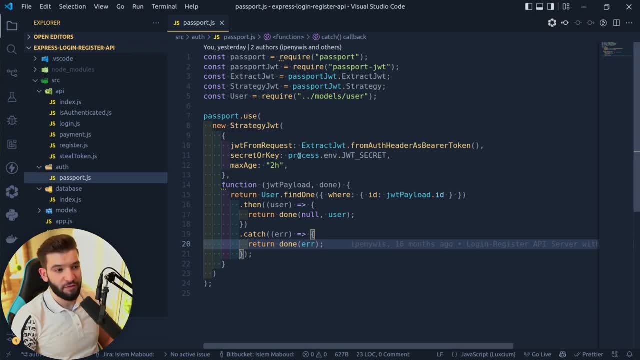 with PassportJS in here And PassportJS, of course, if you're not familiar with this, it's going to allow you just to basically authenticate and use like GWT authentication and do plenty of stuff. So we are using in here to do GWT authentication and to extract that from a 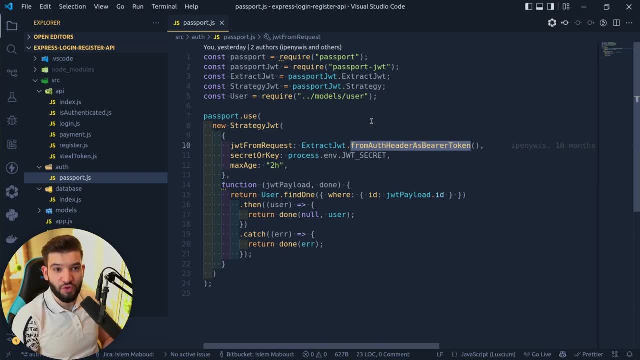 bearer token. So I'm using this as simple as possible. I'm using the local storage. both of these projects right here, like you know, read from the local storage. no cookies are included, just the local storage, And this is the basic way most of people just implement authentication. this: 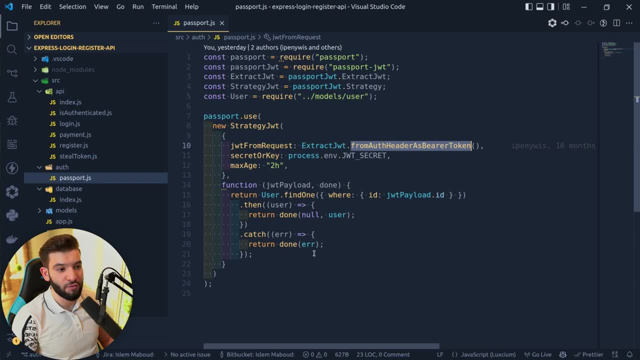 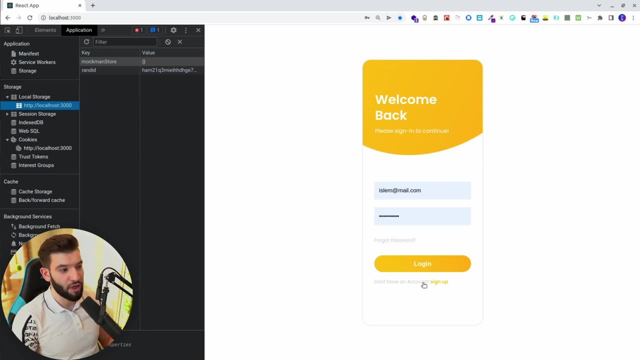 particular way So you can find, of course, the projects and get up in here just to see it yourself. So I'm just going to go through, like the, basically how the project works And for the demo application it's just basically a login, So a login screen here that allows you to authenticate. 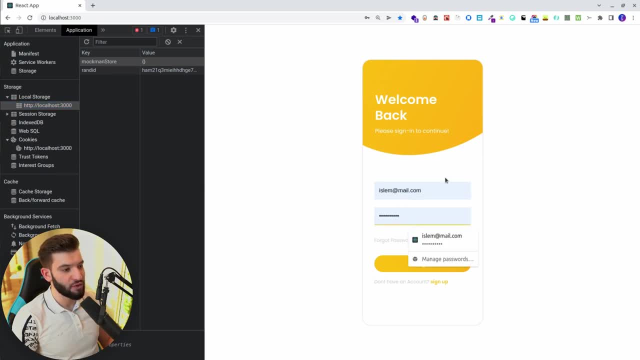 and everything. So once you head over to this, you can just go in and click on to like the email or the password and you can enter that it's going to see welcome back authenticating and it's going to store the API token. So, as you see, this is the API token, this is a GWT. this has been stored into. 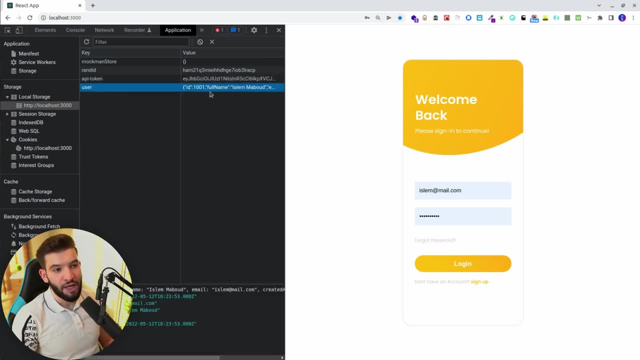 the local storage right For that. we're going to click on the local storage, we're just going to that particular website- localhost 3000. And, of course, some user information in here, which doesn't really matter. So we got just the API token. this is what we need for now, And this: 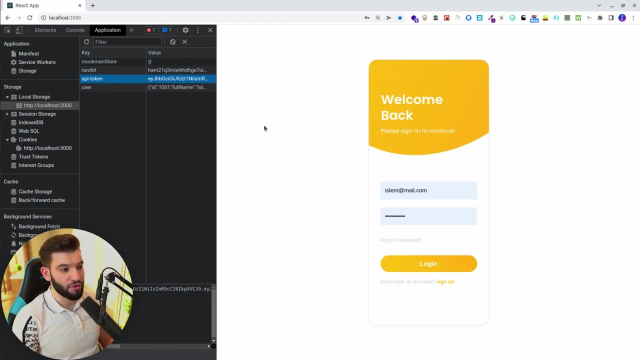 is the GWT. So this is when you're using local storage, of course. And now, once I, for example, go to the dashboard, I will be able to authenticate and the dashboard in here is going to do plenty of requests. One of these requests is going to do is the payment, So it's going to do a request to the 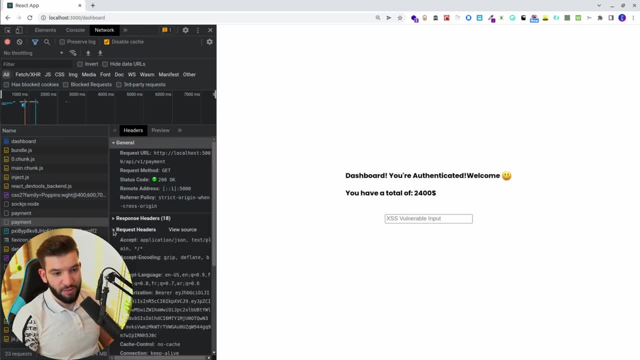 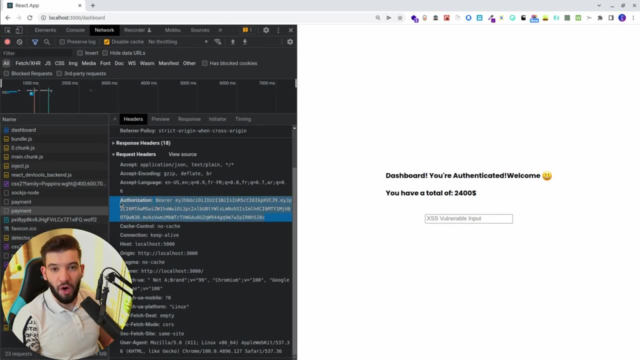 payments API And it's going to send- like not response but request headers. it's going to send the authorization as a header, right as a beer header in here, And this is basically what the authentication works and how GWT actually works- from a local storage. So you send it on the header. 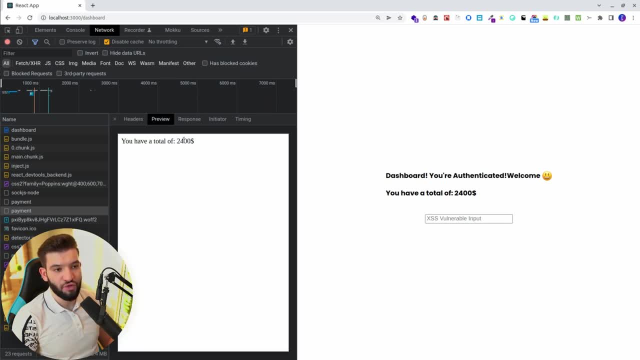 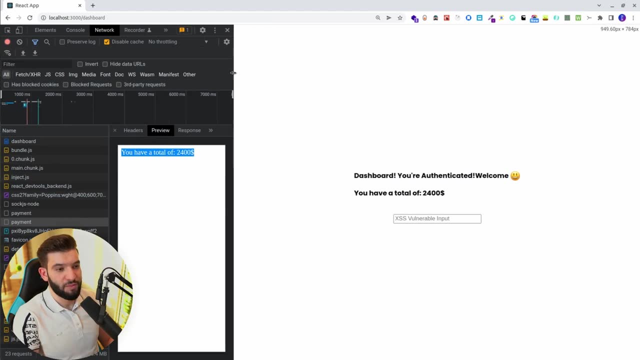 and the server is going to authenticate, is going to return 200, it's going to allow you to access the resource- for example, a payment gateway or payment endpoints- that is protected by that API. Pretty simple, And that's how it works. And if you quickly take a look on the login form in here: 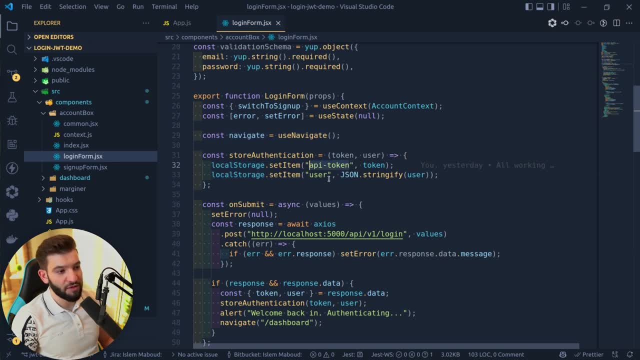 what we're doing is basically using the local storage and storing both the API token and the user, And of course, we're going to do the same thing here. So we're going to do the same thing here, And of course, we're going to do the same thing here. So we're going to do the same thing here, And. 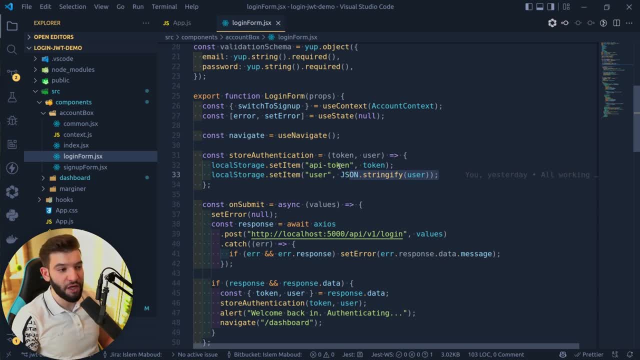 of course, the user in here. as long as you're not storing like sensitive information or like password and encryption keys or anything related to the security side, you know you're just basically good in here. If you're just storing just metadata info, most likely like 90% are going. 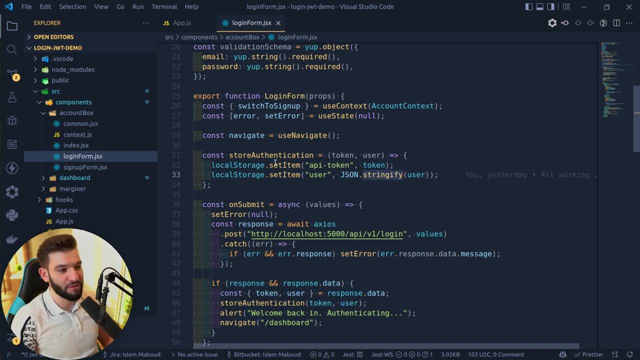 to be good, But you know there's always a 10%. you can be compromised. So there is an API token in here And this is what we care about. This is our GWT token And it's being stored on the local. 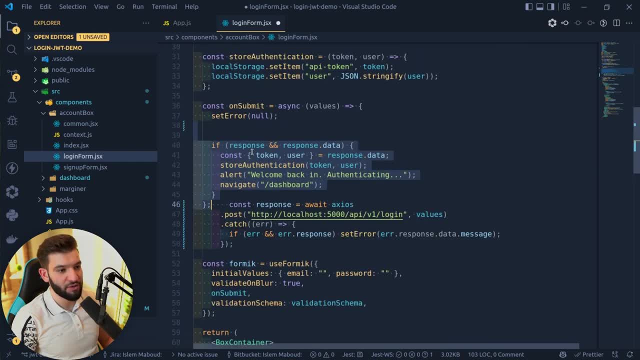 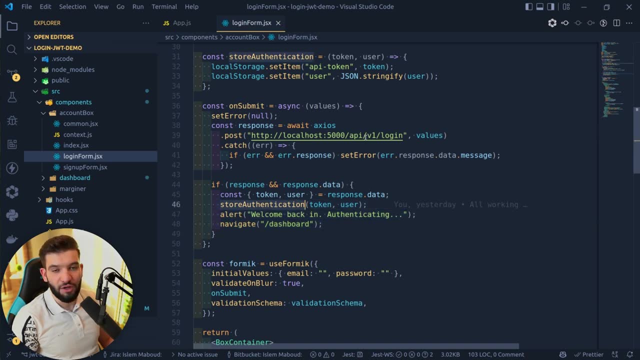 storage. So once you log in, once the submit in here, once the request or response is came back. so once you've got the response in here, of course you're going to just like navigate to the dashboard. whatever you're going to store the authentication and you can call it a day. 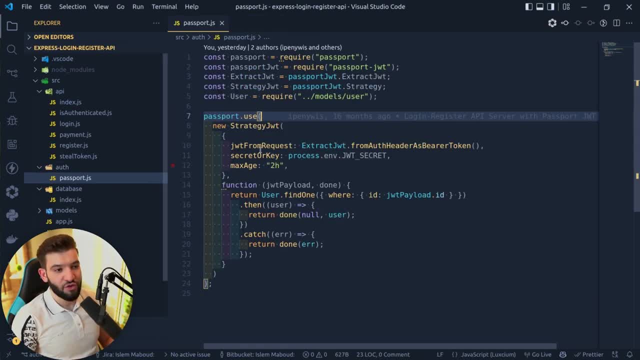 That's the simplest part And that's how it works. If we jump back to the like the server in here, it's basically using the strategy I said before, the password strategy, which basically checks that, or like extract that from the header as a bureau token. Remember, we're sending it on the 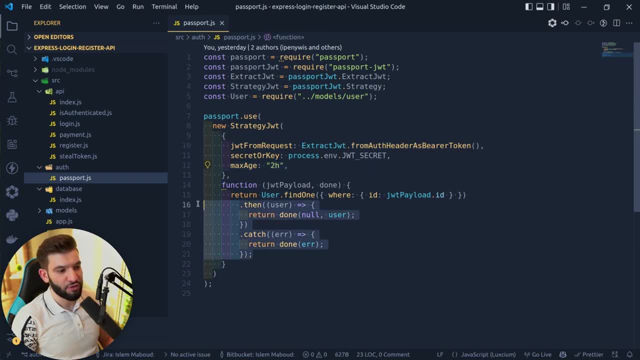 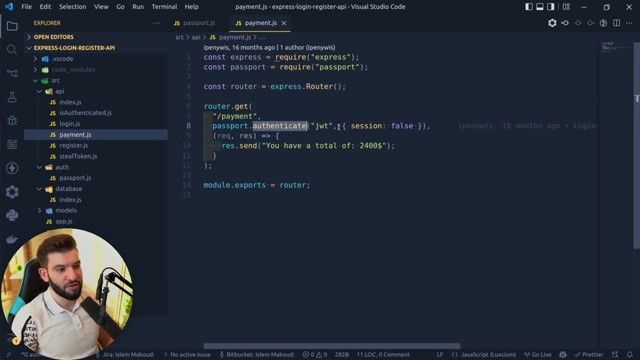 authorization header And of course, it has a max age and everything it looks for the user finds the user that is going to allow you to authenticate with. if you use this particular middleware just to do password authenticate, it's going to allow you to access this because, of course, 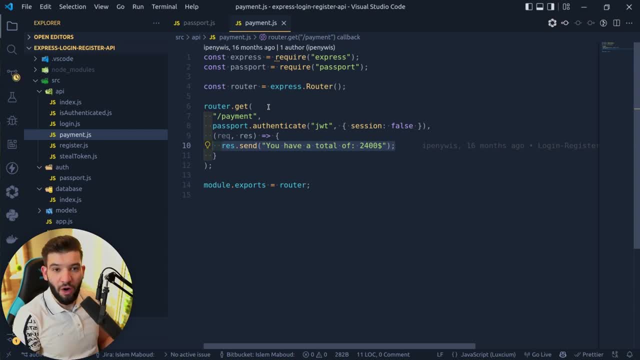 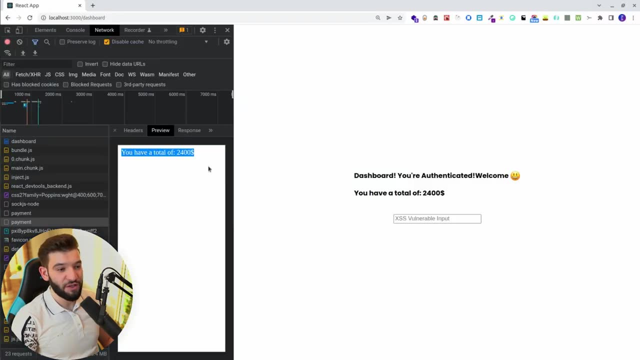 the GWT is valid and everything is working fine. Now why this approach is absolutely bad and you should always, always, avoid this at any cost. So if I jump back in here and I'm just going to give you a quick example of XSS and how this could be very, very bad, 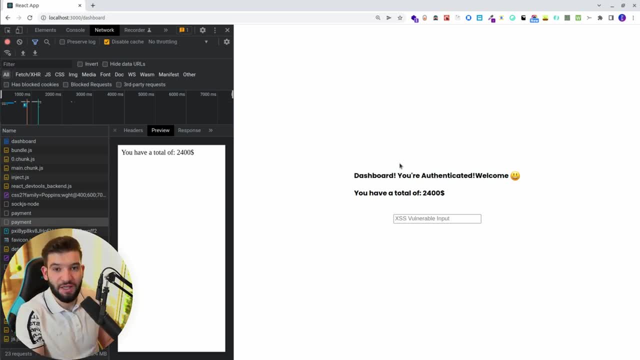 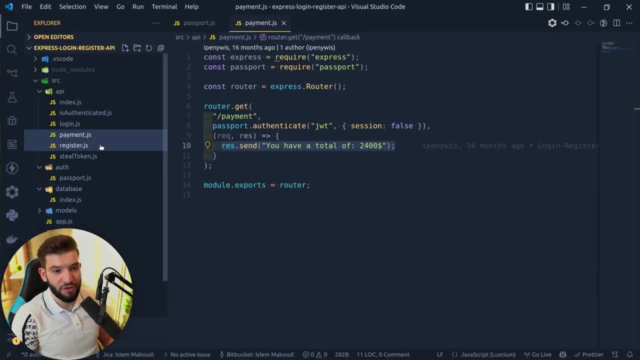 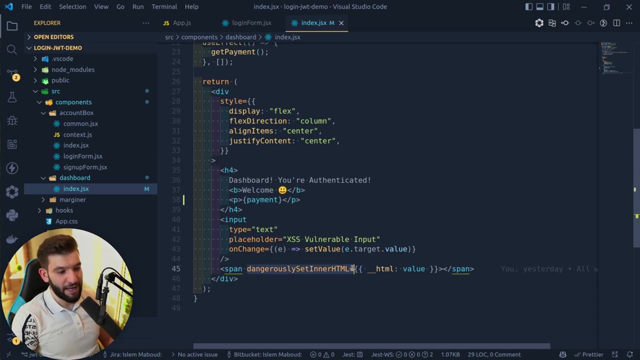 So, since this particular application is pretty small, right, you can't have the XSS unless you implement that. And that's what I did in here: implemented an XSS vulnerable input And if I jump back to this particular input in here, that should be on the dashboard And if you head over, that's just like sets an inner HTML. 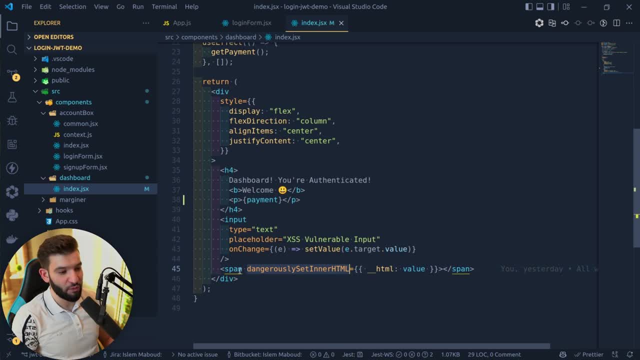 right, Because reacts by default, escapes any HTML stuff by what wants to do dangerously, set inner HTML. you're you just like, have no warranty anymore. So that's what I'm doing in here. I'm just creating this XSS. But if you are having this big application, a medium sized application, 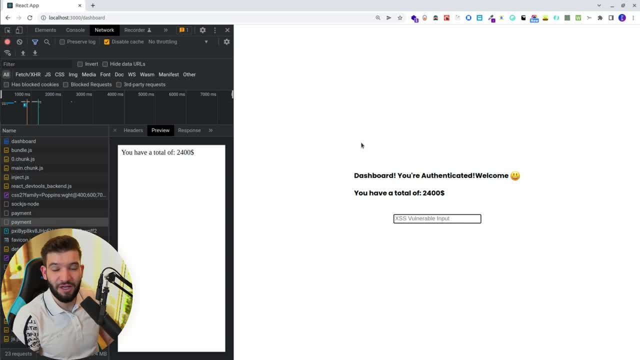 even a small application. you can have XSS anywhere in your side of your inputs. You can imagine how like you can get an XSS and you can actually figure it out. So it's very, very bad to do that And you can always assume your application has an XSS. Okay. 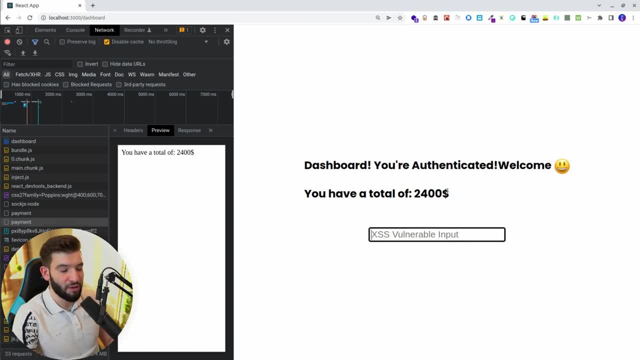 so I have an XSS in here and I have an XSS vulnerable input. I don't care how, but you can execute XSS on your application And that's already care about. So I got particular different payloads in here just to try XSS payloads particularly. So I'm going to try this. 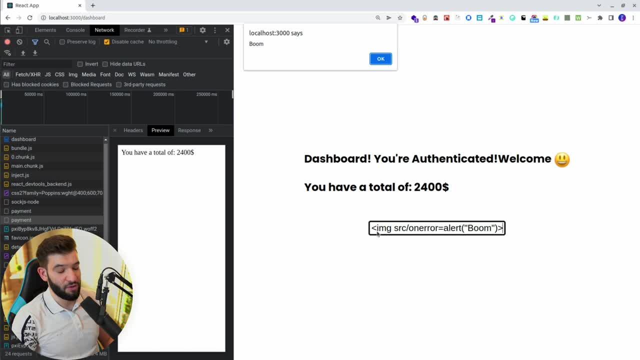 particular payload that's going to run an alert, just to check that is. this one has an XSS and is clear to see me when I put an image in here, as I'll see, and I can run custom JavaScript code and that's what should happen in here. That's pretty good. I just have an alert Now. what can an alert? 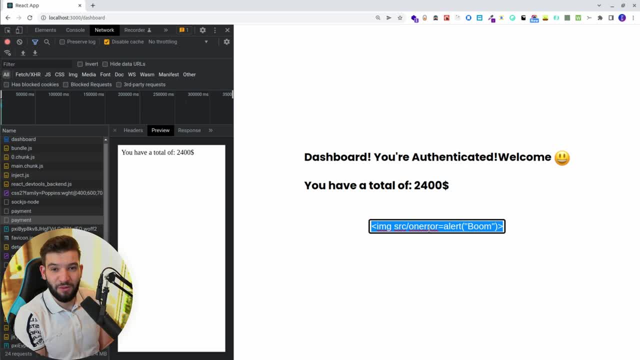 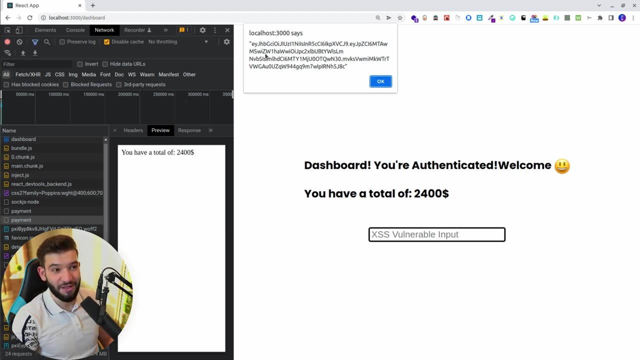 how, like hurt me Because that doesn't sound like really dangerous, because you're just doing an alert. Just, you know, hear me out with an alert. like you can start from an alert, but what you can end on you can have an alert, but this alert can have the GWT token. like that's crazy, that's your. 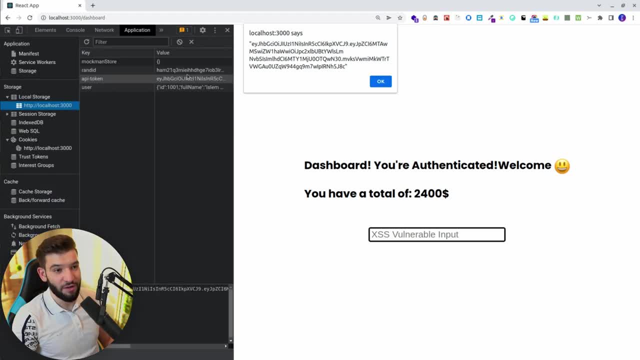 token in here and if you head over to the application right over here, you can find this is the exact same token and anybody can access that token, because they can run suspicious or malicious kind of JavaScript code inside of your application and they can access local storage, because JavaScript can access local storage and 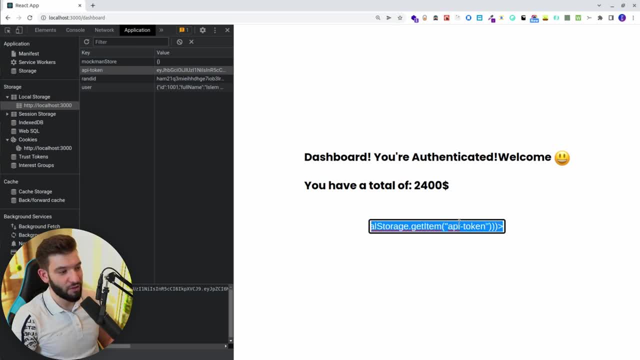 that's a pretty bad bones. So just putting this XSS in here which can run and doing everything, that's pretty bad. I mean, like you can get the local storage, you can get the API token, you can do plenty of stuff. So as long as you can execute, 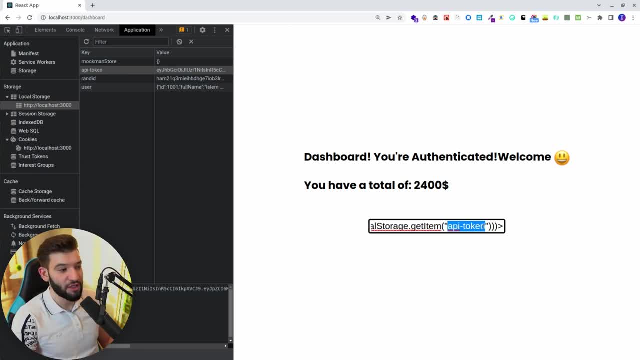 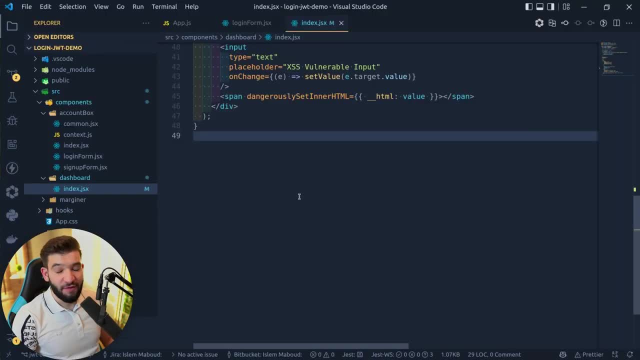 JavaScript and you can access the underlying GWT token, which is the local storage. you can do whatever you want and the hackers can have fun with your website. and I've got another payload that is pretty suspicious and and it's actually you can. it can actually steal your GWT token. you. 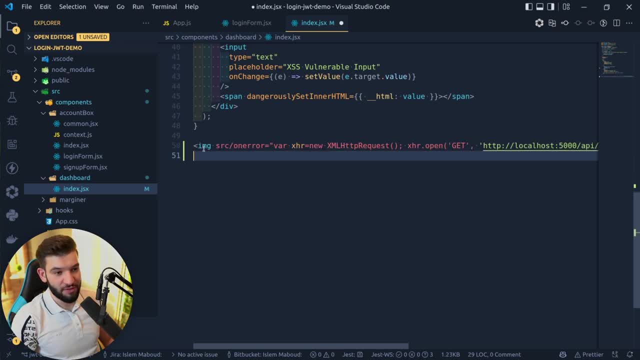 can send it to a server and it can save it on a server. so this payload in here just it's an image again. it uses XSS vulnerability and it does one error. then it just uses XML HTTP request module, it uses a particular API and I've actually implemented the particular or simple API. to steal a token, then, 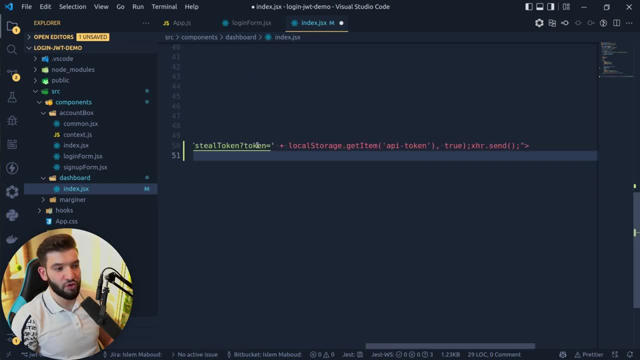 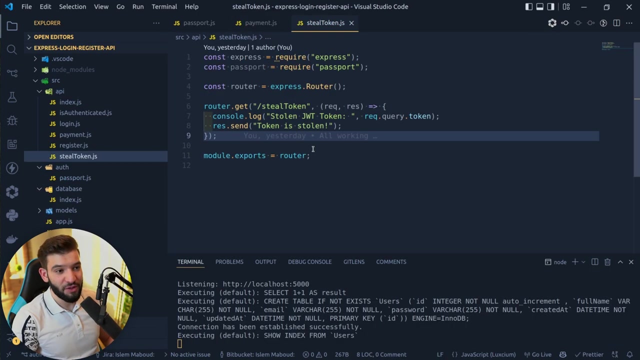 it just like, appends that token from the local storage API token to the token and he adds it to the HTTP request. then he sends that request all just by executing it on your input. and why is that? just because you have your GWT token or local storage hackers can actually do that. if I jump. 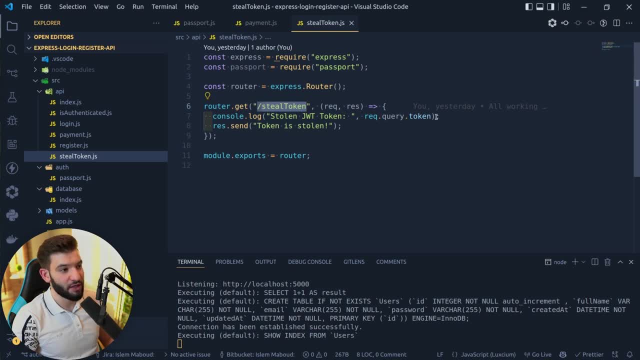 to my server. I got a simple endpoint in here that allows you to steal a token and it can grab the stuff, and this is this is actually very dangerous- and you can just like you can- grab it from a query, you can save it on database and this API- reviewers- can be a hacker's API and it can steal different. 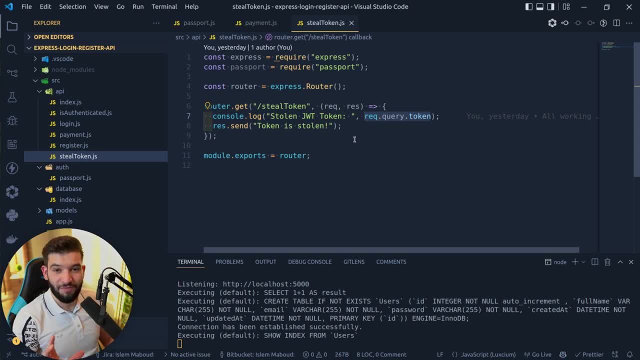 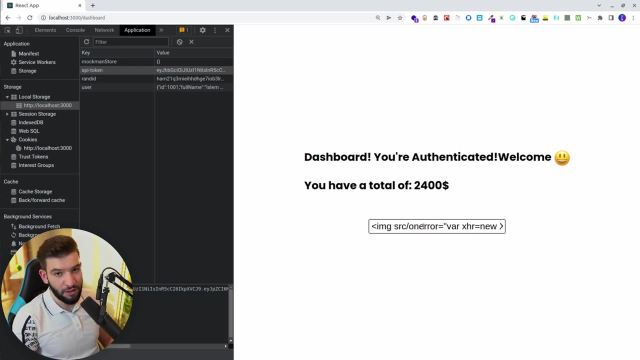 GWT tokens and you can use them for evil stuff. so yeah, keep in mind in this. so let's go and try this particular payload. I've got the input in here. I'm just gonna click on this. I paste today. I see nothing. really like nothing happened. okay, if I go to the network tab, I'm gonna see something. 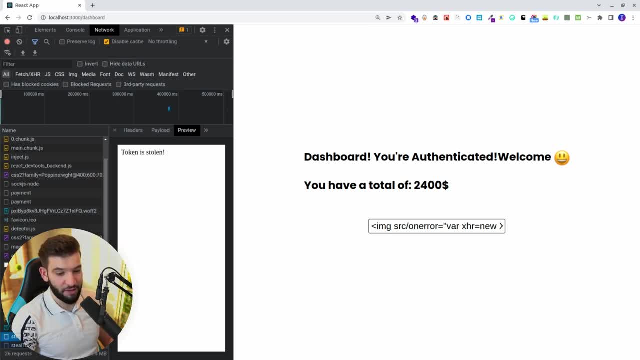 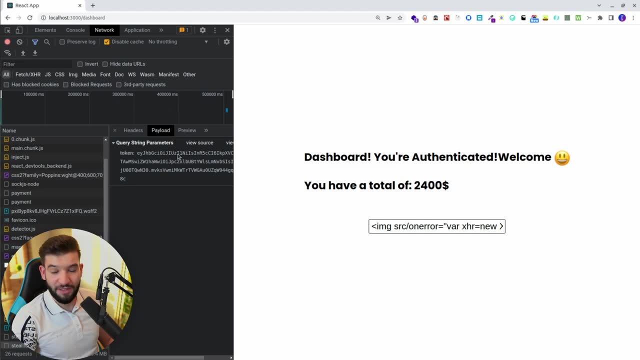 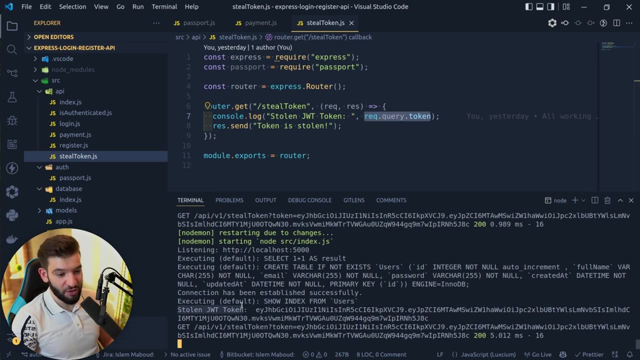 suspicious. there's an like a hidden- some like a hidden network call made and there's token is stolen and the headers are pretty simple but the payload is actually our token. wow, if I jump to the server, if I go to the logs- because I'm console logging this- I got the. 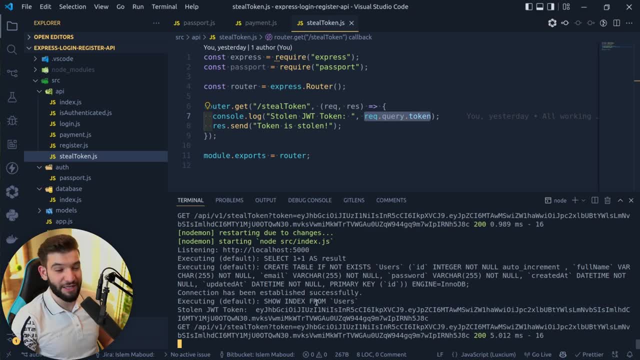 stolen GW token and this is actually the stolen GW token. it's. it's actually. this is what it is and why this particular one happened in the first place. I'm not going to say excesses, because excesses could be like happening in every application, and you can't mitigate excesses, so it's very. 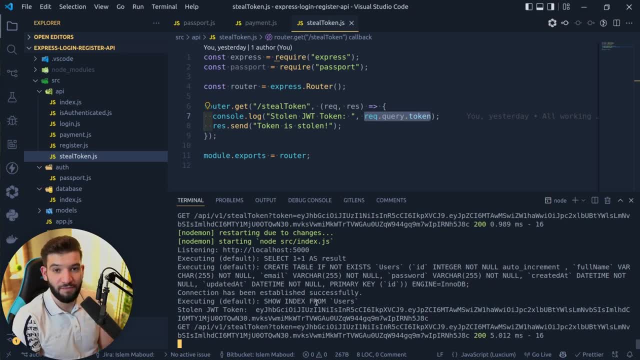 mitigated very hard to fix your exercise, even though you need to find and fix those particular excessive vulnerabilities. you still can't control that unless, or in the other side or in the other hand, what you can actually control as a developer and the easiest way. of course, it needs a little. 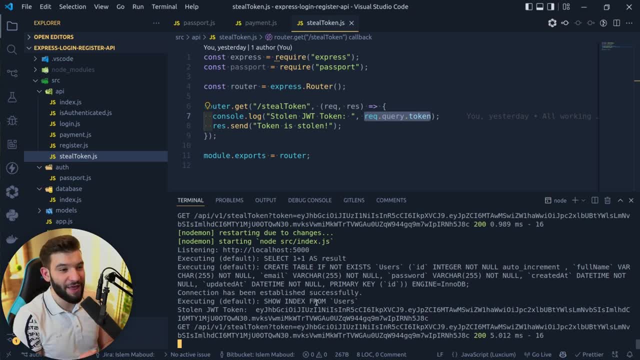 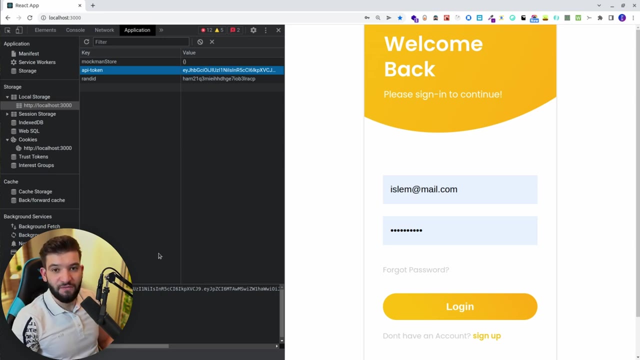 bit of just, you know, changing here and there, but the easiest way and the most actual way to do authentication, to implement authentication, is to use http only cookies. so if you're still using GWT, your local storage, the first thing or the easiest part that you can mitigate just right away is 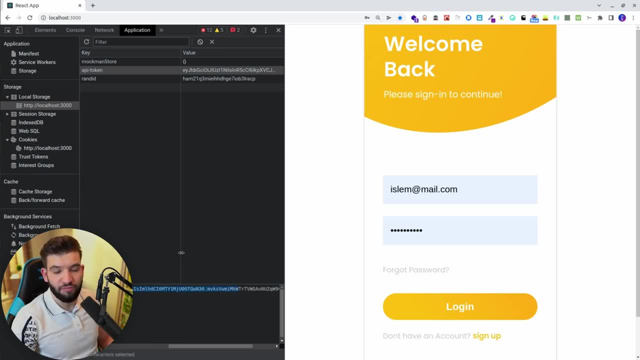 actually to make these GWT tokens expiry date just like too little, like two hours or maybe five hours, something like this, something or like a timing window that cannot affect that much. then later on you can actually change it to http only cookies. so just like a quick resort, you can. just you know. 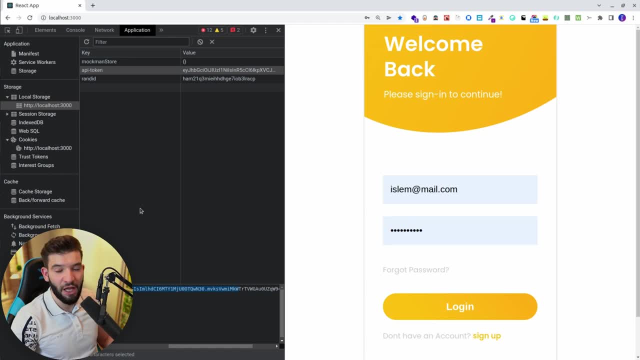 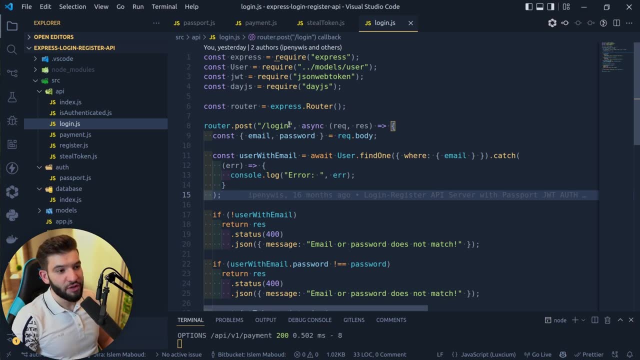 change the expiry date or expiration time for this and just make it a lot lower. now for http only cookies in general and particularly http only cookies and particularly, for example, in here, the login in here, this: I changed the projects in here to use http only cookies now instead of I'm sending. 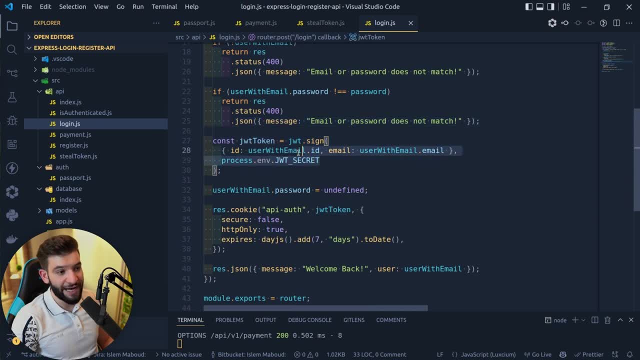 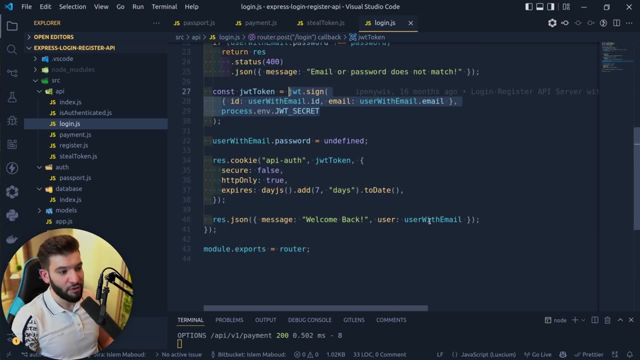 the GW token on the header. as you see, I'm doing the GWT token, I'm signing the GWT token and everything, but instead of sending it back on a header or sending it back as a response, I'm not doing that. I'm just sending the users data, without a password, of course, and I'm sending that gwt as. 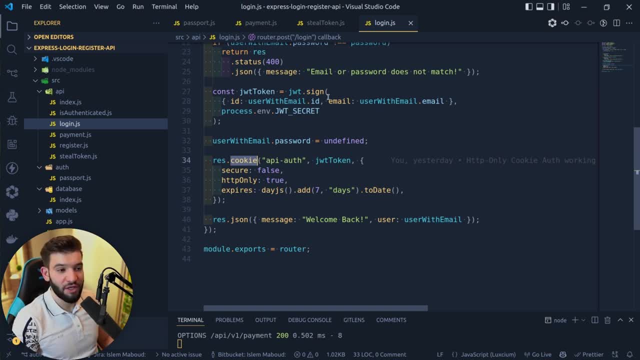 a cookie and, of course, if you're not familiar with how http work or http cookies is, once the server sends back a cookie, the cookie is going to be automatically set on the underlying browser for the particular local or for the particular domain that you know the cookie owns. so that's particularly where it's going. of course you can set secure in here if 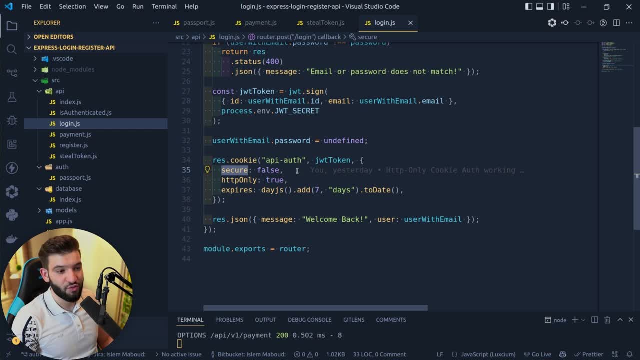 you're http or https and SSL, and because I'm just running this on localhost, I'm putting this false, but make sure to put it true if you're in production. and I'm putting http only, and this is a very, very actual, crucial approach to do for cookies- not just cookies, but you have to do. 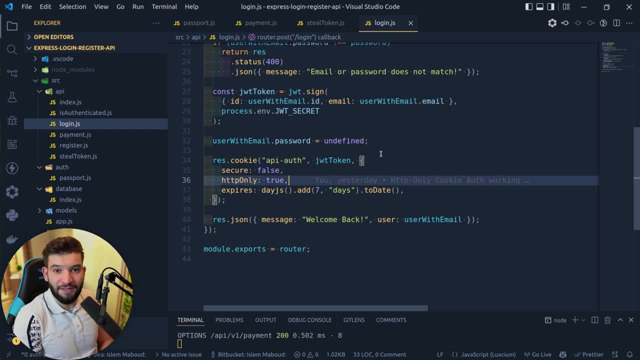 http only cookies, because http only cookies cannot be accessed by JavaScript. so no JavaScript code can access the http only cookie and the cookie is going to be sent automatically by the browser when particularly making any requests to the underlying the mean that the cookie has. so the browser is. 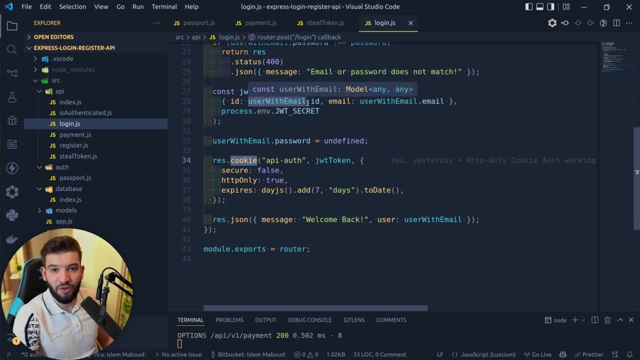 going to take care of handling the sending the cookie and the server is going to read the cookie as it does for the haters. basically just need to add just you know, cookie parser and that is it. okay. that means you can actually run no XSS or no excess of vulnerability can allow you to access. 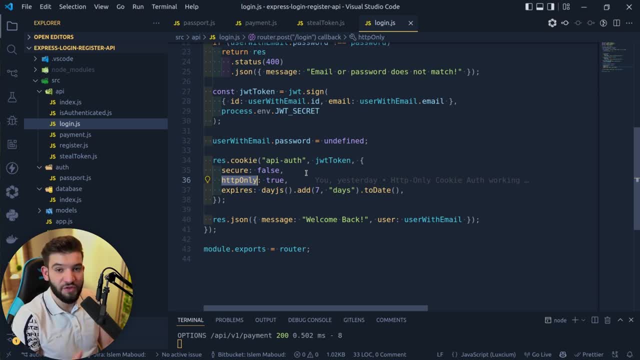 that cookie, which means you cannot do like session hijacking. you cannot steal the GW token because the cookie cannot be accessed by the JavaScript, and that's actually a very good approach. so, simply, here I'm just doing the cookie in, here I'm just returning the cookie and that's what it is. so you 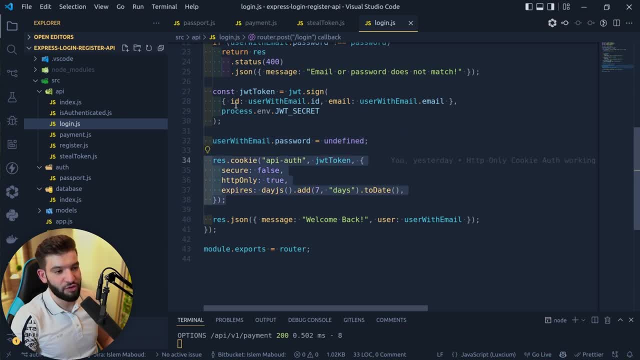 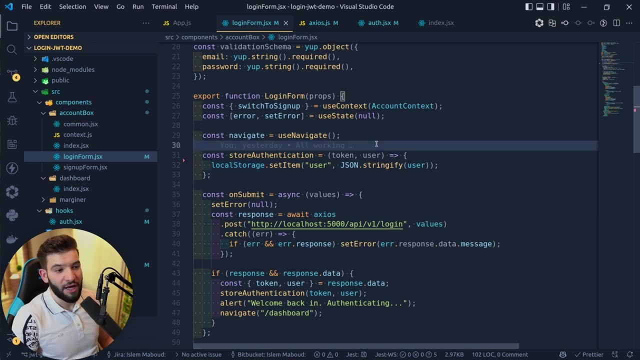 like you don't need to go through the details of how that particularly works. so just, you got the cookie in here. of course, in the other hand, in the front end in here particularly, I'm not sending it on the local storage anymore. I'm just going to leave that to the server to set the cookie, because 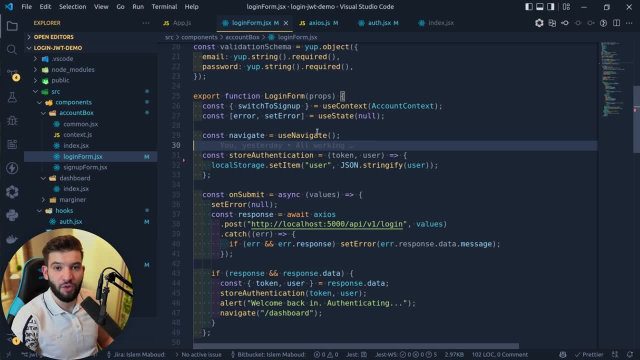 the server is going to be, you know, be able to return the cookie, and the browser is going to send the cookie automatically for you. so you don't need to do anything, just save the user in here. whatever meta data you need, and the authorization token or the GW token is going to be handled by. 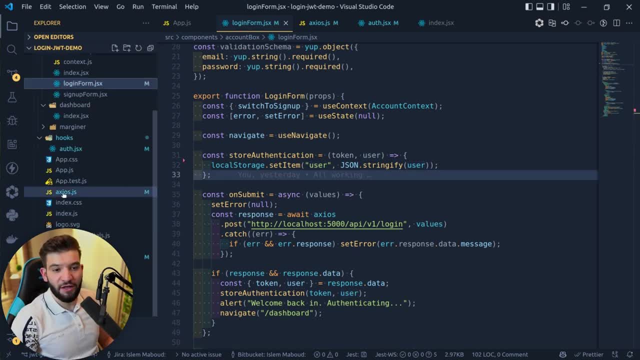 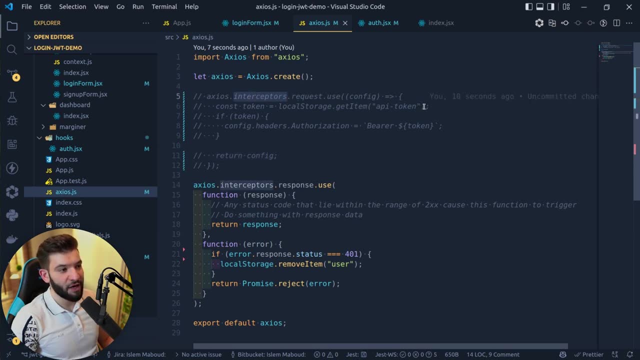 the server in the browsers themselves, pretty easy. and if I take a look on the axios interceptors, because before we were using the actual interceptors to intercept every single request and add that like add that from API token from the local storage and add it to the authorization header, so to allow that now I 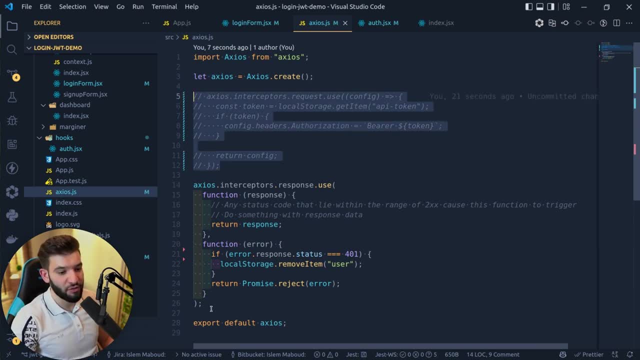 commented this code because that's now needed. the cookie is going to be sent automatically by the browser and when, like the response is coming in here. when you have like an authorized, I'm just removing the user in here because that's all I'm using for authentication and because I can't remove. 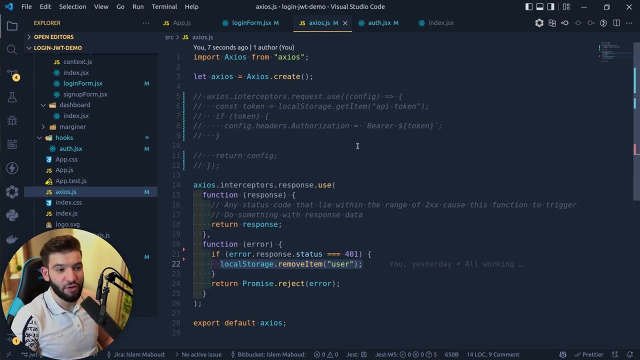 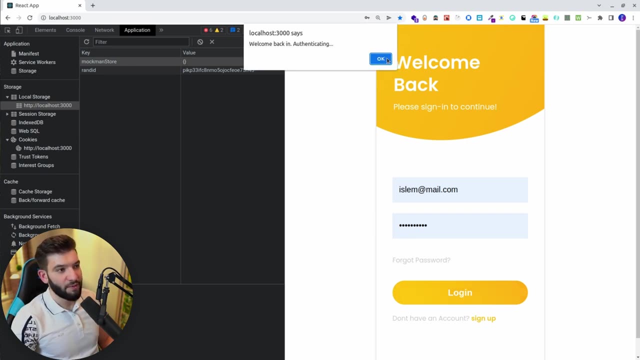 the cookie. the cookie needs to be cleared by the server. so that's a pretty good approach now if I jump back to the application real quick in here. so I tried not to log in with cookies and it's been only cookies. they click enter. I'm going to be authenticated and get no luck, you know. 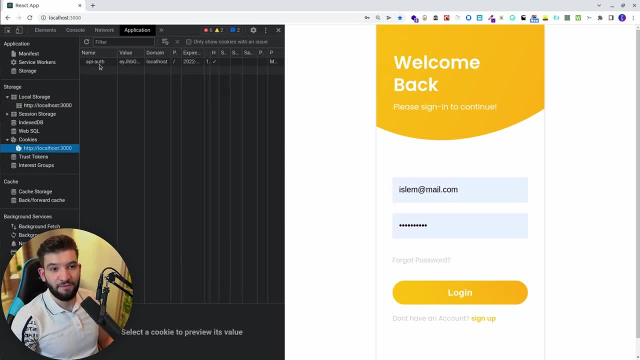 API token saved all the local storage. but I head over to the cookies. I'm going to find a new API auth and it has a cookie, it has a domain, it has expiry days and plenty of stuff and plenty of you know details and it's just going to be working fine. so if you head over to the dashboard in here, 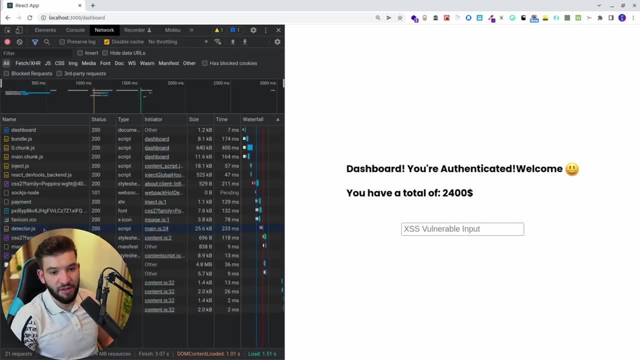 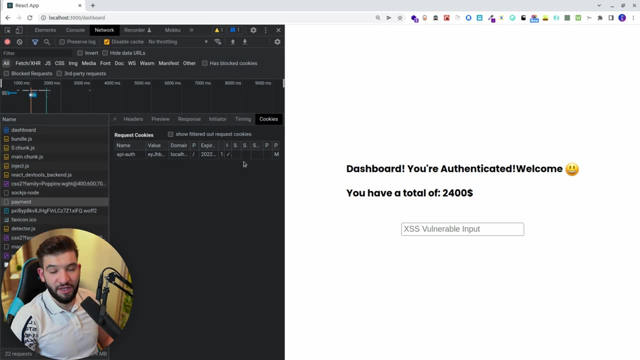 you're going to be authenticated. it's going to allow you to access- you can access the payments in here if I go to like the payment round. that's going to work and you're going to find cookies that are sent like request cookies in here. it's going to send that every single time. the browser. 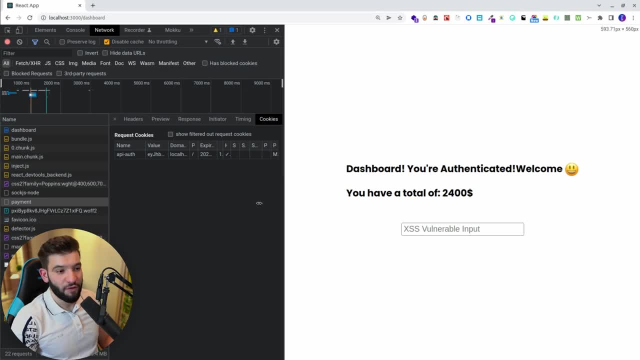 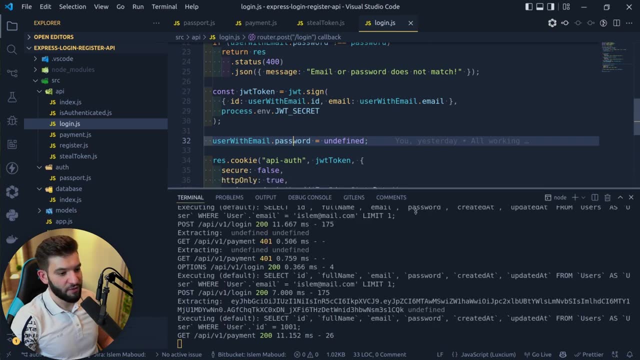 knows and everything. so that would work fine and, of course, in here for this particular example, if we try to do any XSS right, I've got the XSS in here and I've got my server in here. so this is my server. I need to you know to be able to see if I can steal anything now. 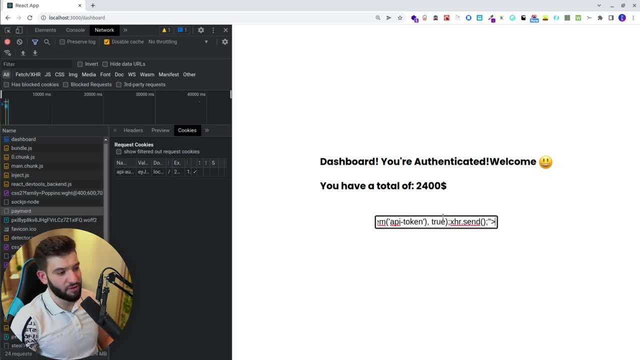 if I, you know, put that in here, the actual is, you know, because it's XSS, it can be still be called. but if I take a look on the token, the payload it's null. because you have no access to this, the local storage is not accessed anymore and you cannot access cookies, HTTP only cookies. and if I 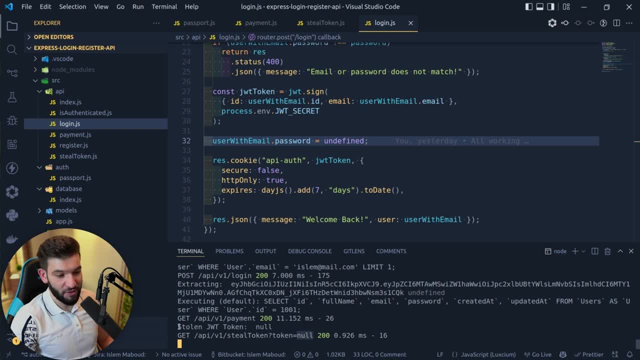 take a look on this: the token stolen and it's going to be called as null and, as you can see, stolen or stolen GWC token is going to be null and they can no longer steer your GWC tokens, and this is the best approach to secure GWC tokens in the first place. also one: 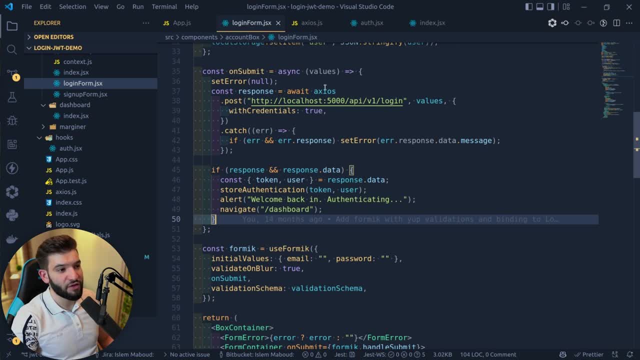 other thing you need to keep an eye on. so when you use cookies right now with Axios or with fetch, so what you want to include is actually, you want to include with credentials. you can include it per request or better, you can include it as a default. so you can do Axios defaults with credentials and 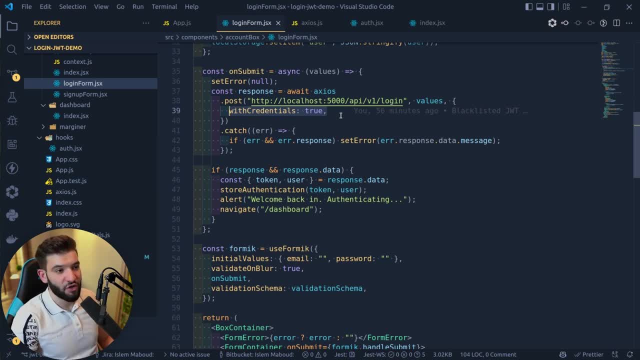 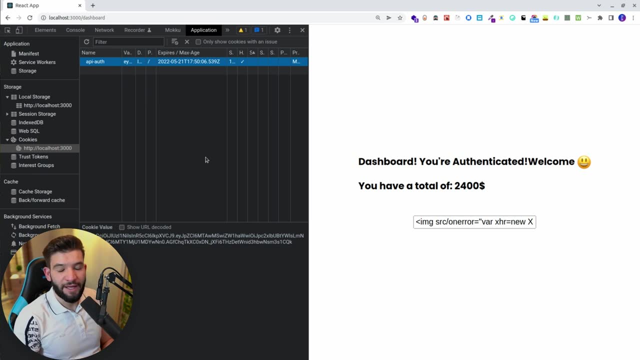 then this will allow it to send and set cookies and everything. so make sure to do that when you change from local storage to, you know, HTTP only cookies. and the other very awful thing I completely disguise about using GWTs is actually the ability to invalidate or blacklist a particular GWT in a 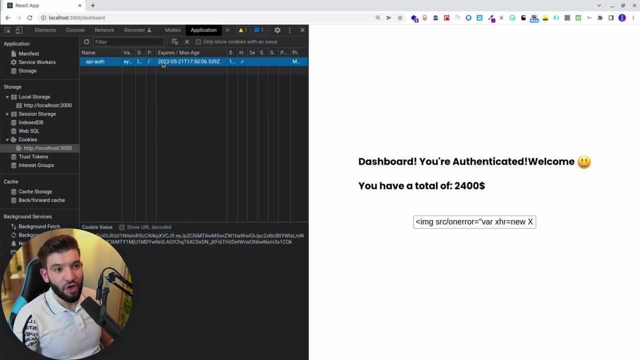 particular type. so, for example, in here you got a GWT right and you've got an expiration time for that GWT- like, for example, this one is from seven days from now- and you won't be able- like the server won't, won't be able to unauthenticate or won't be able to delete and 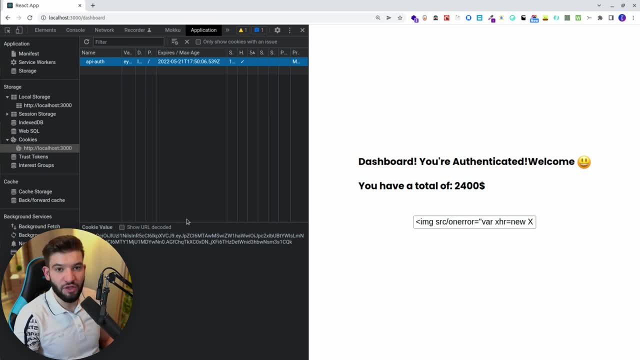 block this particular GWT if anything happens for that particular user, for security concerns or anything in in that particular time. so you won't be able to do that like only. this can only happen once the expiration time is ended, because GWTs are stateless and you cannot keep them on the database. 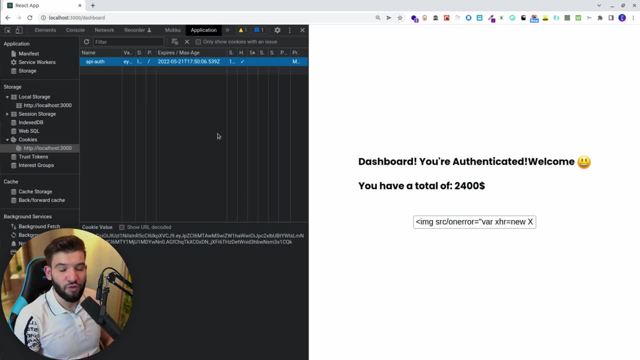 or something so likely. there is a particular way and they can make them, or they can make them still be stateless kind of stuff, still not include them or save them on the, store them on the database, but rather you can store them on a Redis cache, like an in memory cache or just like even in disk cache, because Redis is super. 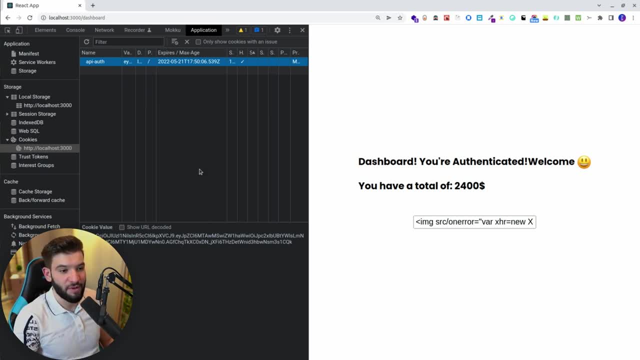 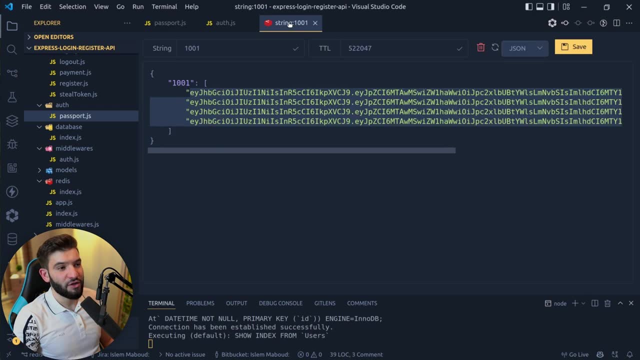 super fast and super powerful and not going to be storing that much of information. you can be doing it on Redis in here. so, for example, right here I got this particular example. it uses Redis and of course. so what I do in this one is actually I use Redis to store like an object, the key for this. 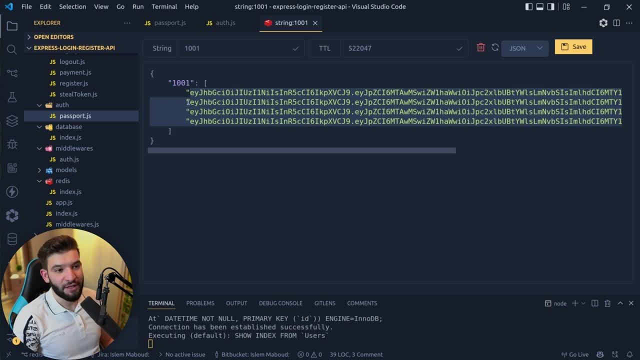 GWTs that the user got before and they were blacklisted. so any GWT is going to be added to this one is going to be blacklisted and the server won't allow it to access that. of course, we need to add a couple of different stuff, but it's actually pretty, pretty simple and pretty easy, so I really 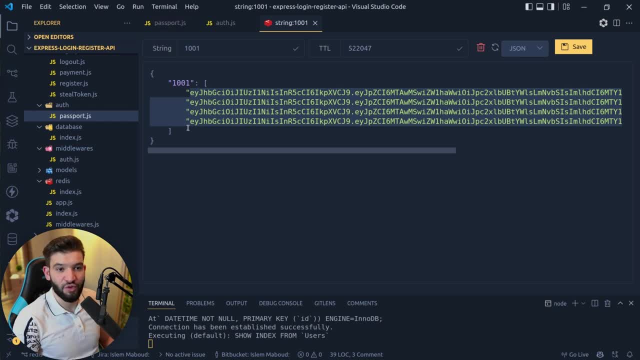 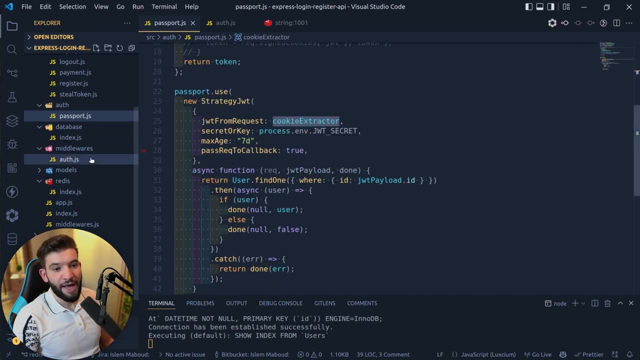 advise you to go to this reticle repo to check how that is implemented. I'm not going to go into all the details, but that should be pretty simple. so we got the same thing, we cookie structure, we got the GWT and I'm using the same thing. what one another thing in here I'm adding is actually a logout route. 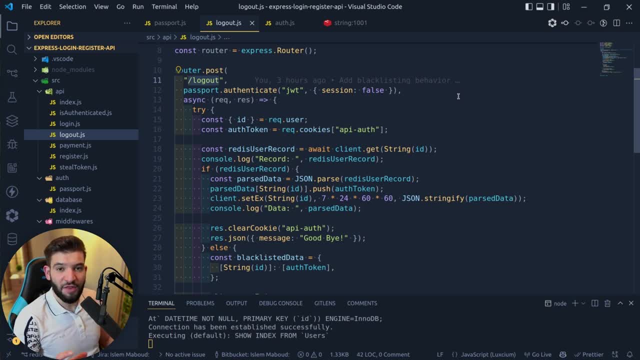 logout button and the request is sent to log out. I want to take this particular GWT of the current user and store it on the Redis so just to make this as blacklisted and nobody else can use GWT because it can no longer be generated and who like if the GWT was stolen before or anything compromised. 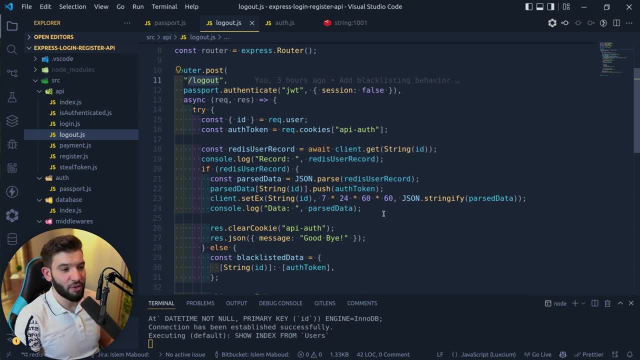 about that GWT. you can just make sure that GWT can no longer access that because the user logged out and everything. and of course you can have different types of different ways to including the blacklist in here. but just this is. this is a super simple example of how to do it. so once the like, you know, once the logout, in here I'm. 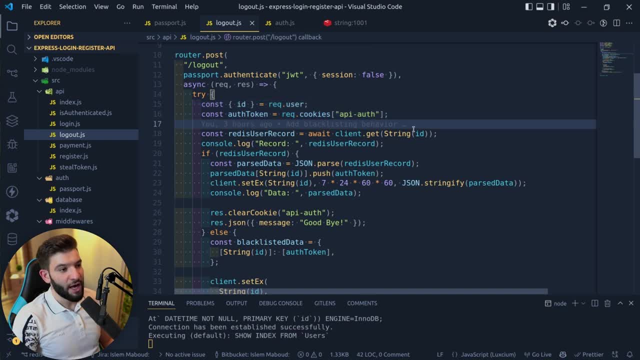 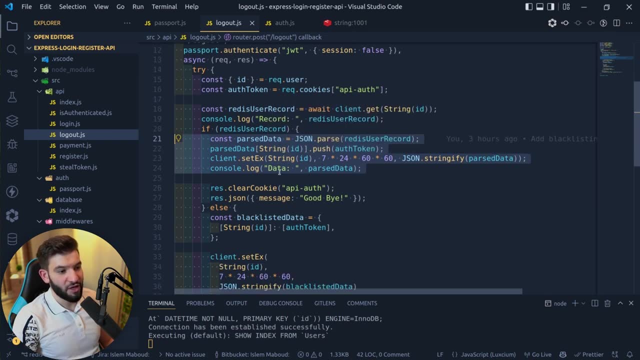 going to authenticate to make sure there's a GWT. I'm going to grab the GWT, I'm going to access Reddit in here to make sure if there's already an user and of course, I'm going to save that users uh, particularly, or save that new like token in here by just looking to the user and saving it if there. 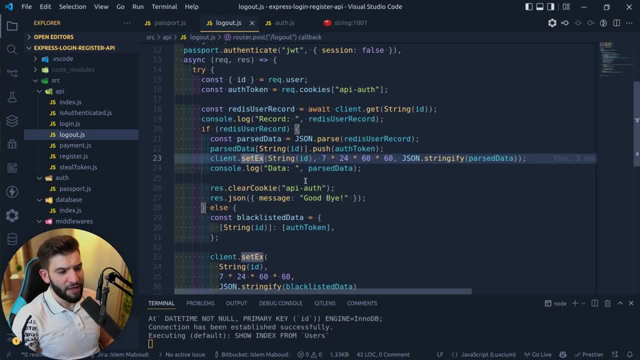 is new user, I'm going to create a new record for it and so on and so forth, and and that's basically what it is, and of course I'm going to clear out the cookie. so I'm going to do response: clear the cookie, the API off. 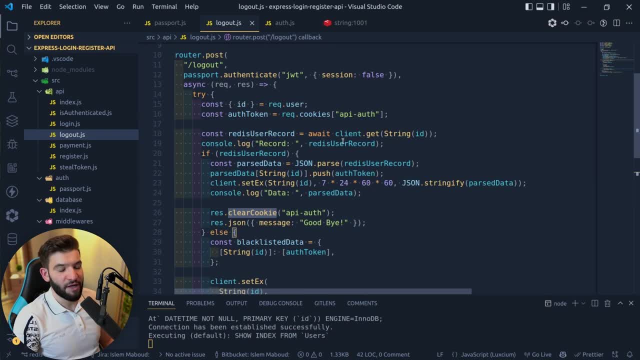 on the browser so it can be cleared out for this particular user and everything would be working fine. in the other hand, this is actually the- you know the way to add it to the actual Redis cache, and there is another middleware created in here and this particular middleware is going to check. 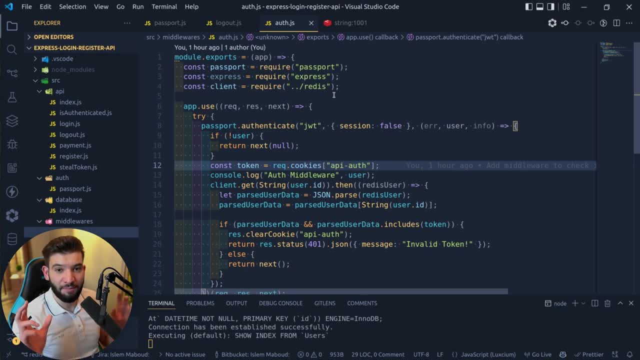 every single request. if it has an invalid, or it has a blacklisted gwt or not. so if it has a black listed gwt, it's not going to be allowing it to access the server. it's going to return 401 and authorized http. you know response. 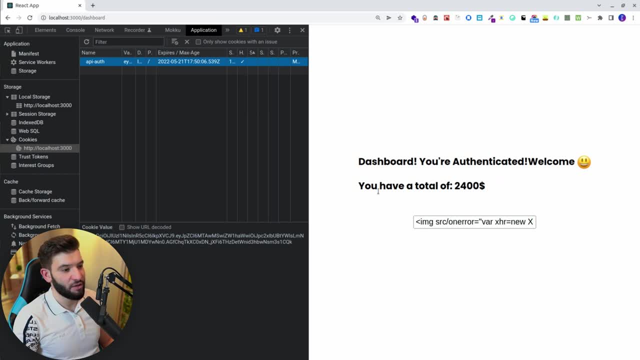 otherwise it's going to allow it to access through. what we can do is actually you can. you know you can log in in here, for example, like I'm going to grab this particular cookie value in here, or what I can do, particularly just a little bit better. I'm going to go to axios, right or sorry, I'm. 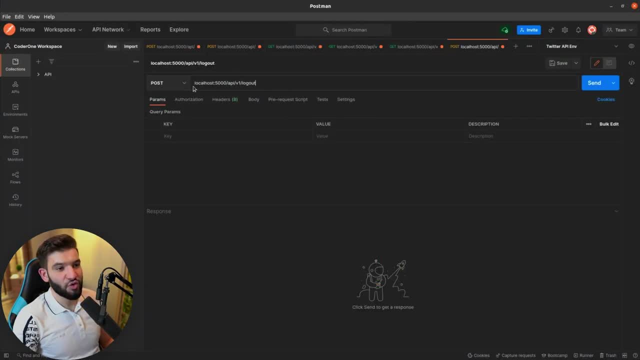 going to go to postman and postman in here. I'm going to close this, I'm going to go to log out, right, and I'm going to try to do that. so, for example, I'm going to be able to log in first. I'm going to click, I'm going to log in and send the password and everything. and here, postman, where? 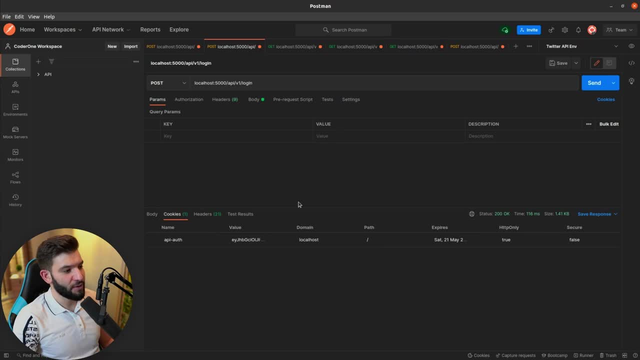 it's located in here and the actual name and the value are going to be kept in here and it's going to be, like you know, keeping the actual cookies. so whenever you do another request to the same domain, the cookies you saved before are going to be sent throughout that request. so, for example, in: 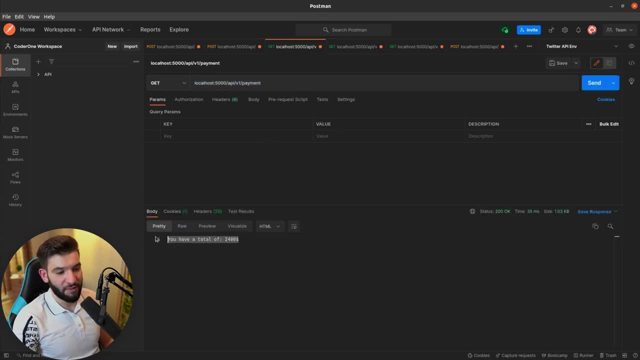 here the payments. I can do payments and it will be able to access the payment. I'm going to get that. you know I'm going to get still get the cookie and everything, but that's going to be working fine. so that's a pretty good approach. now let's go in and try because, if you remember, I'm 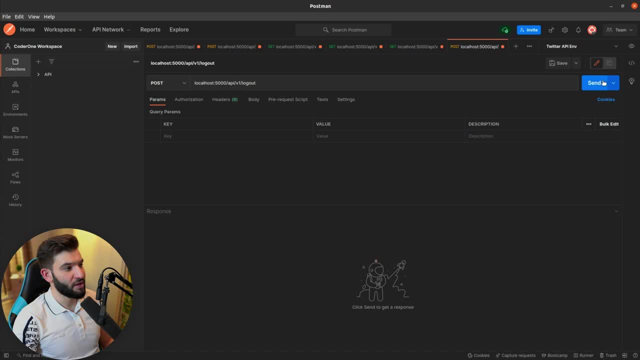 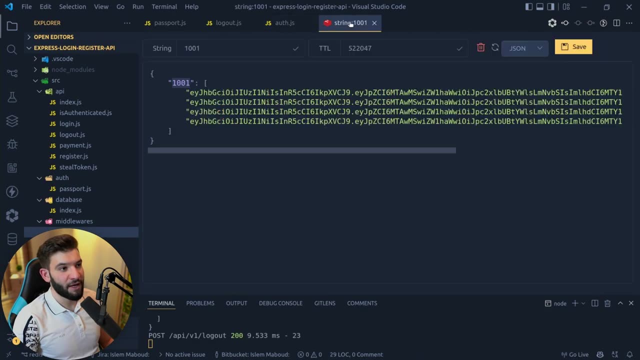 going to go to log out. right, remember, I'm going to log out in here. I'm going to use the same token. I click on this. it says goodbye. that's pretty good. cookies are cleared. there's no cookies back. if I head over back in here to redis and if I refresh, excuse me, there's a new token got added and that's. 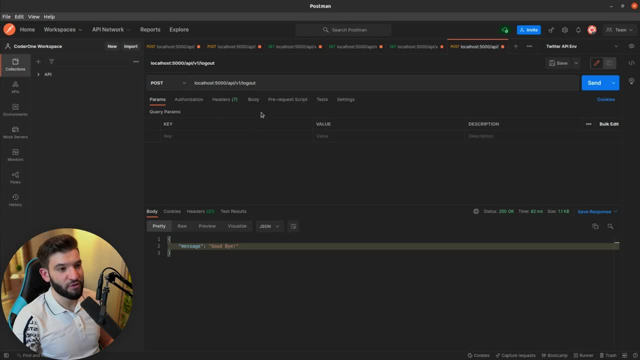 what it is now. it's actually blacklisted and if you try to go back to postman in here and if you try to head over to the payment API, try to send a request, you're going to have an unauthorized right because you're logged out and all those tokens and everything are. 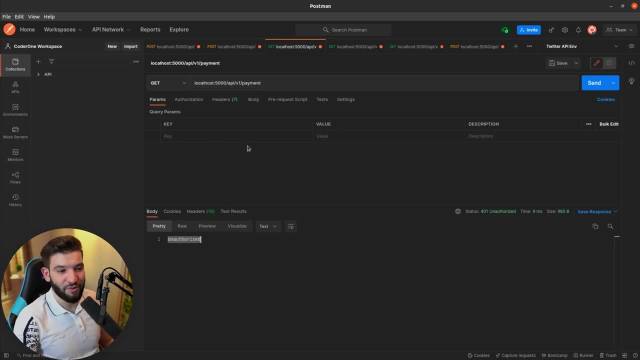 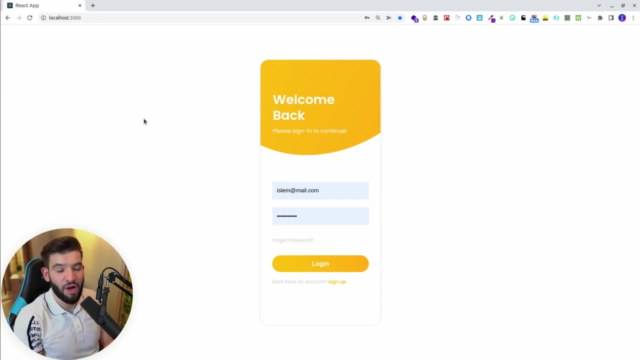 you know, removed, even though the cookies are removed, so that would work absolutely fine. so, anyway, guys, thank you guys for watching. we hope you guys enjoyed this particular best practices for gwt and how to secure APIs or how to secure a react application and browser application, and 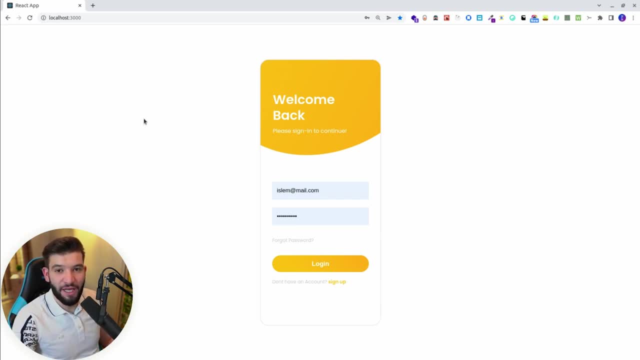 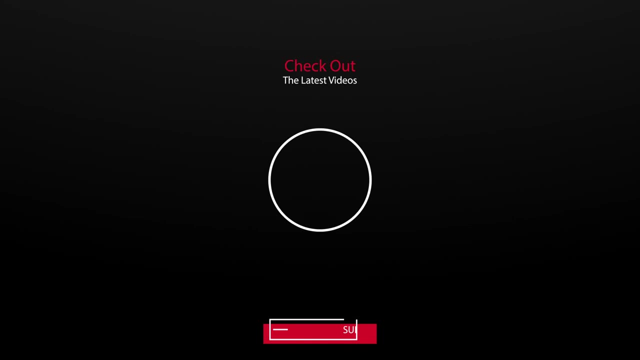 to make it absolutely like a standard secure application and make it absolutely work. fine. so, without further ado, guys, hope you guys enjoyed and catch you hopefully in the next ones. so